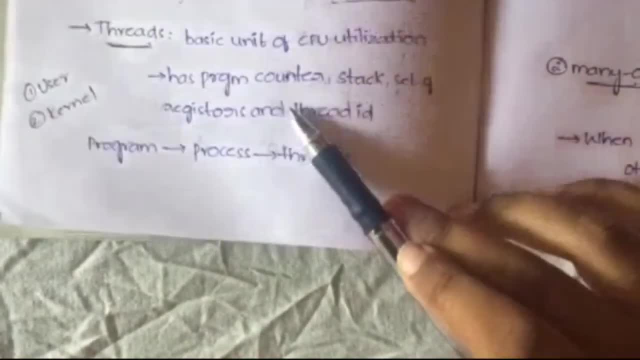 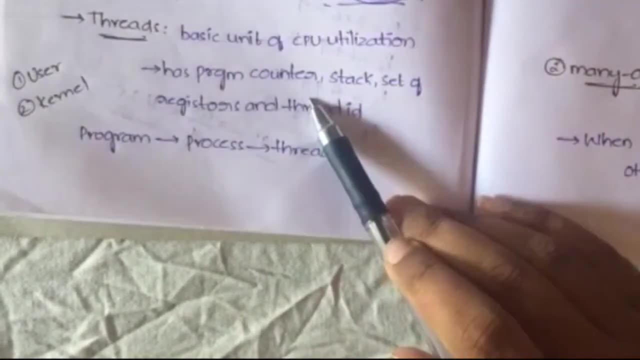 part. okay, And every thread has program counter, stack, set of registers and thread ID. A process has a process control block. right In a process control block it will be storing all the information: process ID counters and so on. So in a process control block it will be storing. 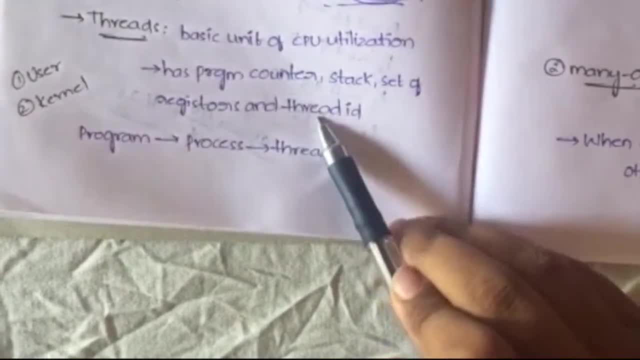 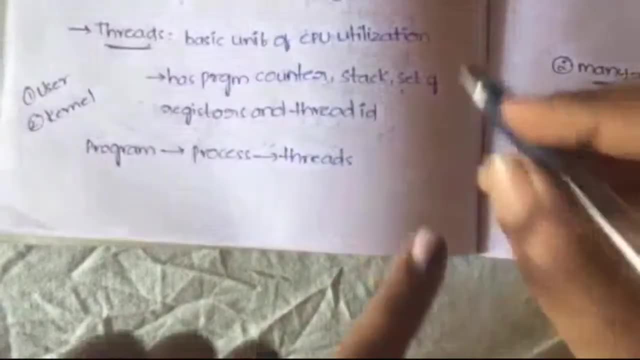 memory files and all those things. In the same way, even a thread will also have a program counter. Program counter is nothing but next which thread will be executed? Suppose thread T1 is in execution right now, Then next which thread will be executed? Suppose if T2 is to be executed next. 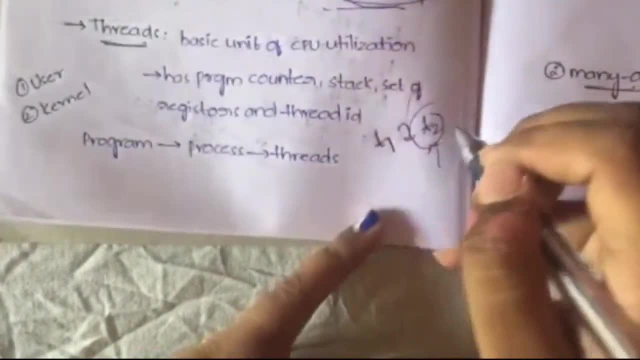 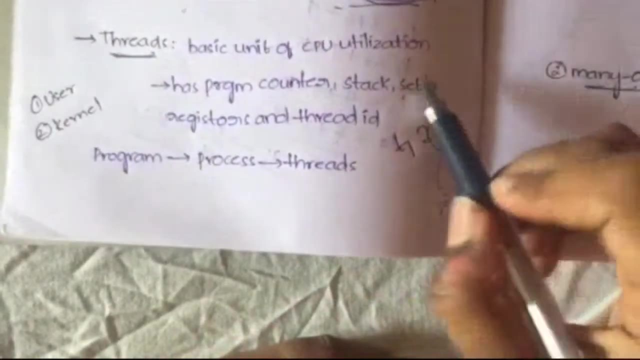 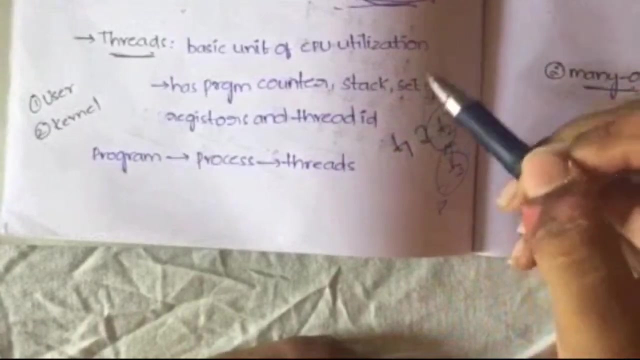 then the program counter will be pointing towards T2.. Or if T3 is to be executed, next program counter will be pointing towards T3.. That is program counter. okay, Next is stack Stack. stack is nothing, but it is used for storing your files, storing memory, and all Next is set of. 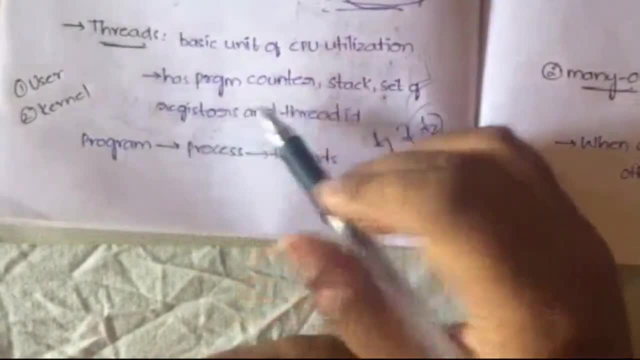 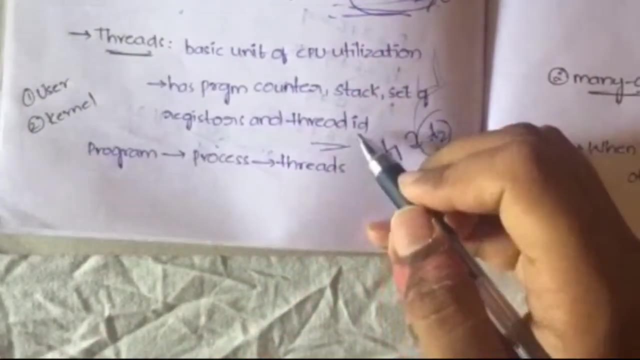 registers. Registers is also same purpose. It is also used for storing the memory, storing the data. Next is thread ID. ID is a mandatory thing for everything. Even human beings have their own ID. That is the reason: in order to identify a particular thread, it will be having a thread ID. 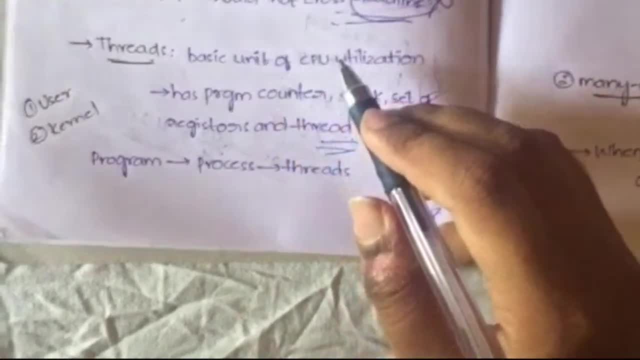 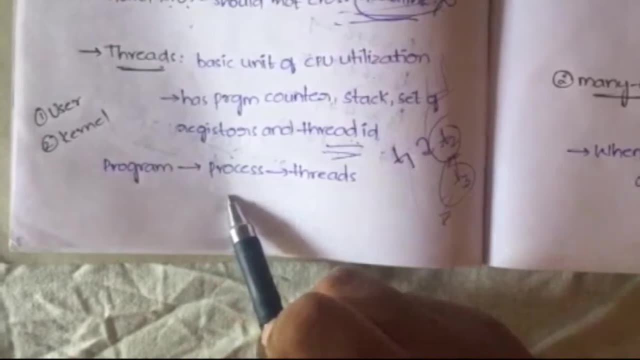 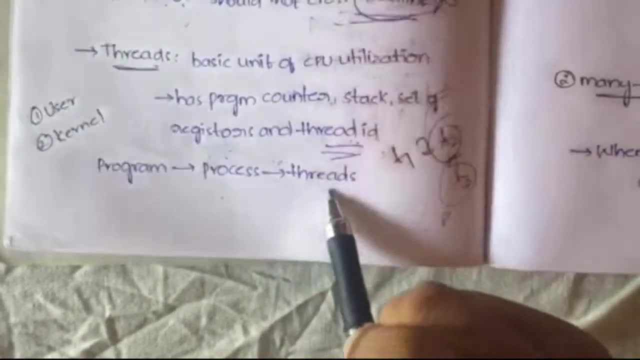 okay, This is the concept of thread. In simple words, you can say that a program will have number of process, right? We know that In the same way how a program has number of processes, the process also will have number of threads. So to understand threads, 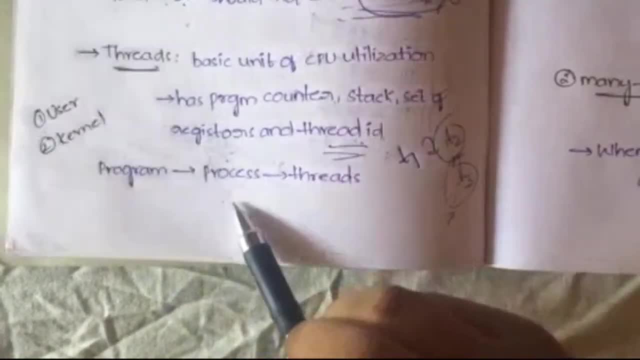 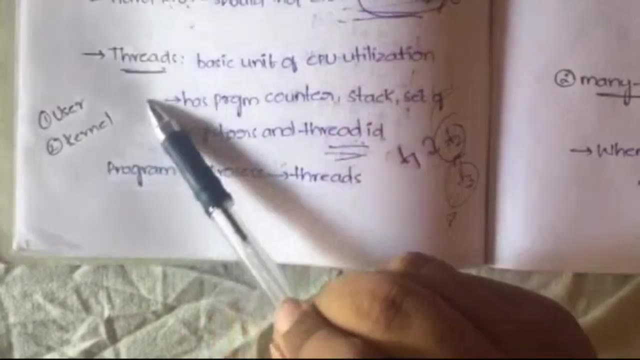 easily. you can remember this program like how program has process. In the same way, process has threads. okay, Again, in threads you have two types of threads: user thread and a kernel thread. Whatever the user mode, operations are there, all those will be. 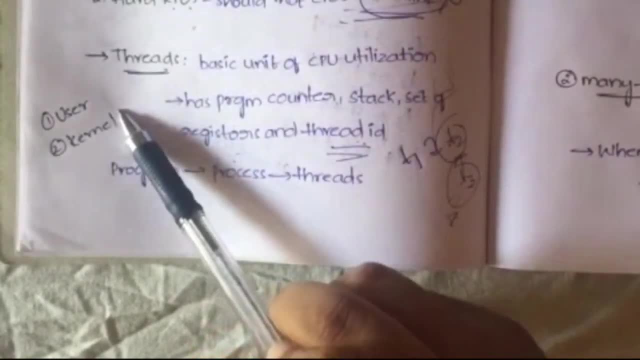 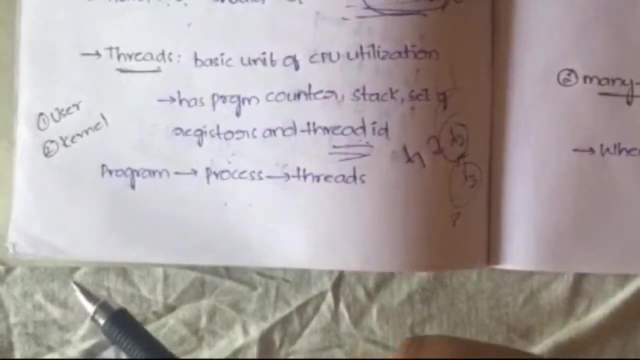 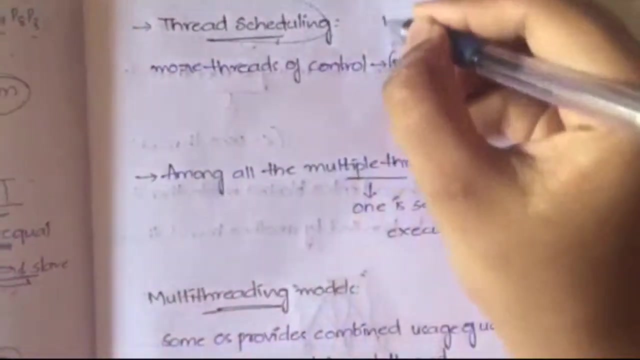 performed by the user thread. Whatever the kernel mode operations are there, all those will be performed by the kernel thread. okay, Now let's learn about thread scheduling. You are clear about threads now, right Now. what is thread scheduling If you have a single thread? 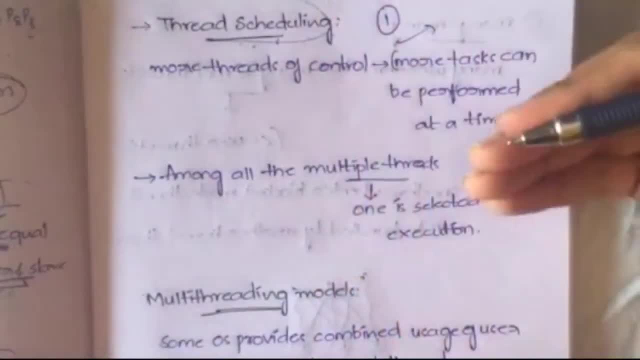 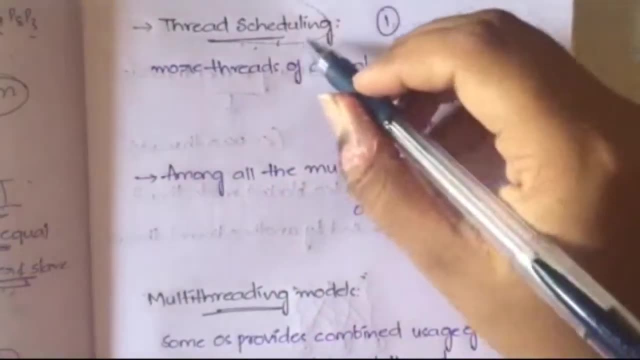 then it is easy. You can directly send it to the execution. It will complete it execution and come back return the output to you. But if you have many threads, like in multiprocessor, you have many process right Here. if you have many threads you can send it directly to the execution. 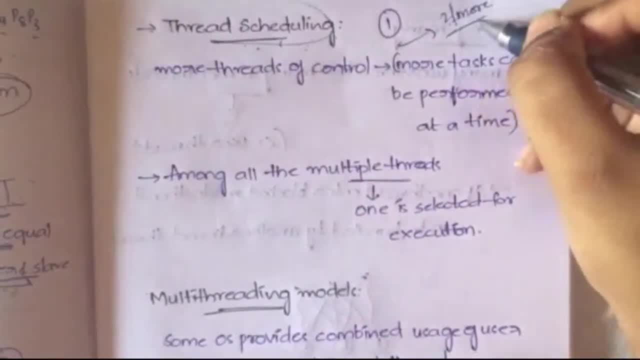 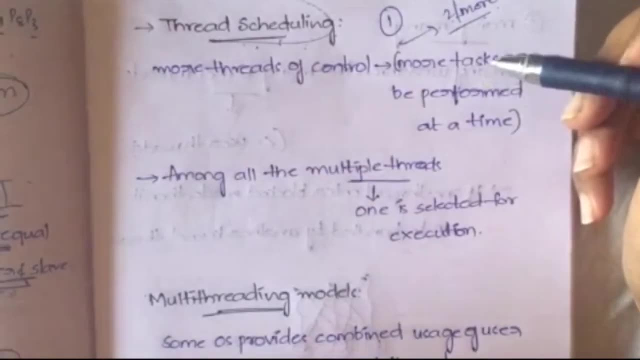 threads: one, two or more threads. if you have two or more threads, then you have to schedule those threads also, like how you schedule the process. in the same way, you have to even schedule the threads also if you have more threads, of control, that means simply threads. if you have more threads, 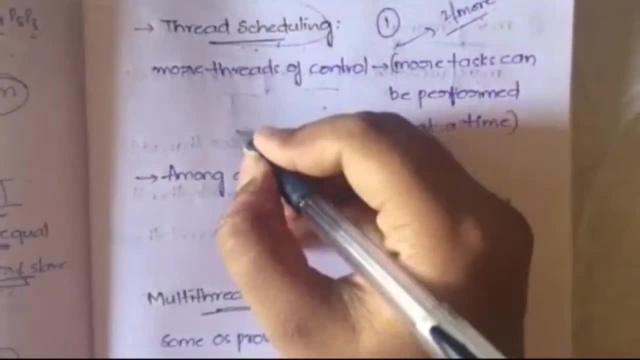 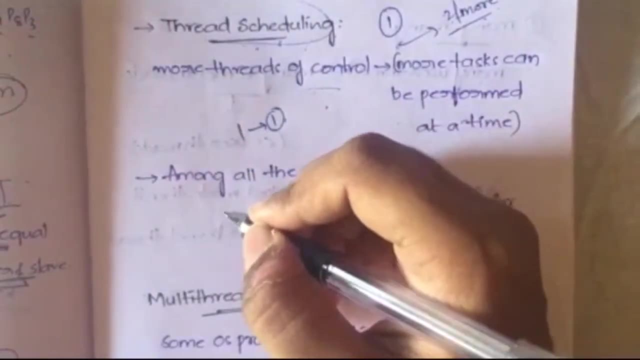 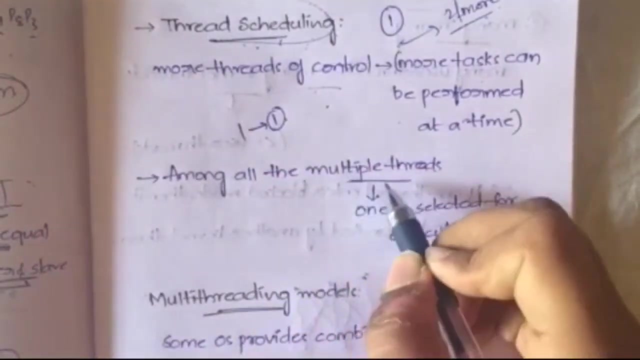 then you can perform more tasks at a simple time, because one thread will perform one task. if you have many threads running parallelly, then you can perform many tasks at a time. that is the reason why you need the concept of multi-threading. okay, so among all the multiple threads you have you. 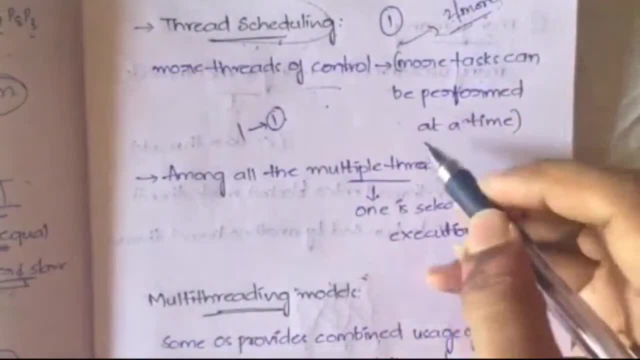 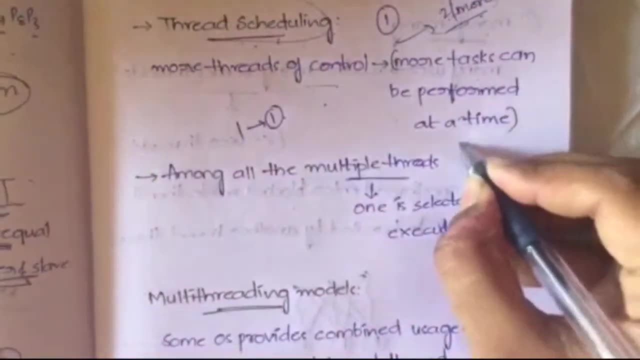 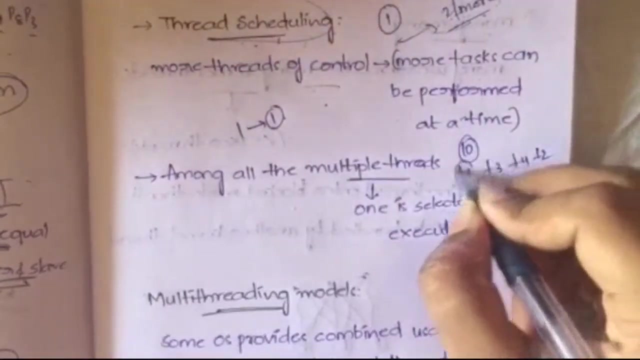 i already said you, if you will be having two or more threads sometimes. so among all the multiple threads you have you have to select one thread for the execution, the next another thread. suppose you have 10 threads, then first you have to execute t1, then t3, then t4, then t2 and all. so this order. 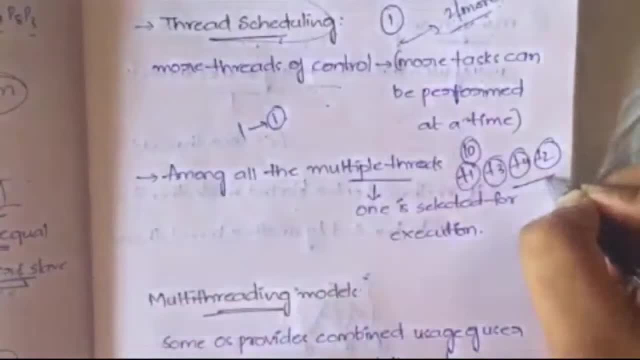 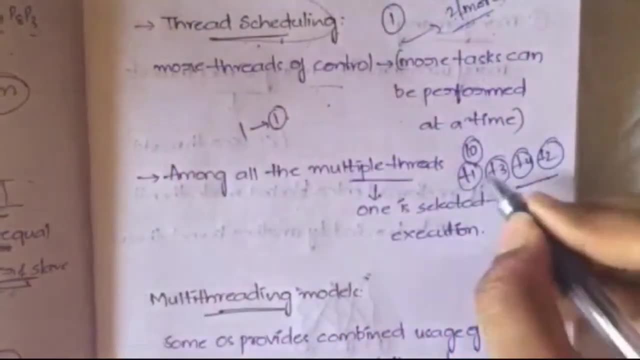 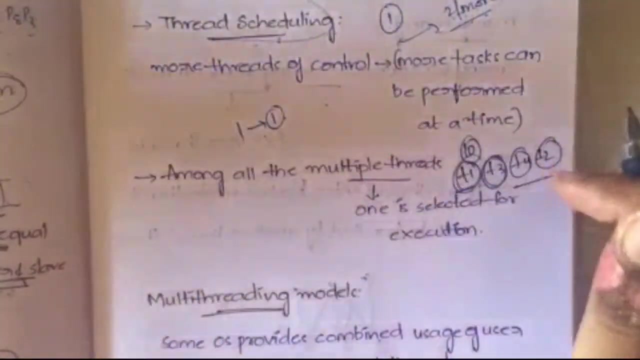 this. deciding this order is nothing but scheduling. thread scheduling is also same to process scheduling, but in process scheduling you will be scheduling the process. in thread scheduling we will be scheduling the threads. okay, clear about thread scheduling right now. in thread scheduling we'll have some multi-threading models. 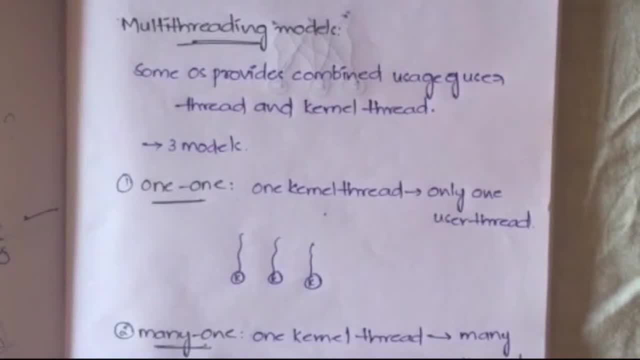 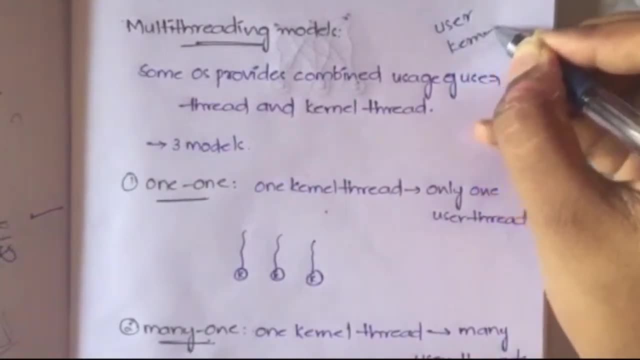 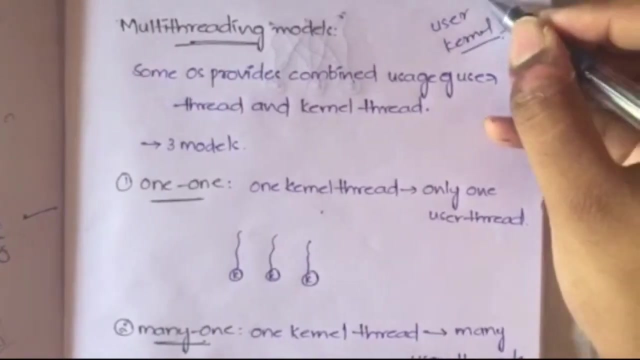 now let's see what are the multi-threading models that we have. as i already said, you you have two types of threads. one is a user thread and another one is a kernel thread. so, combined use- in some operating system you'll be having the combination of these two: user threads and kernel. 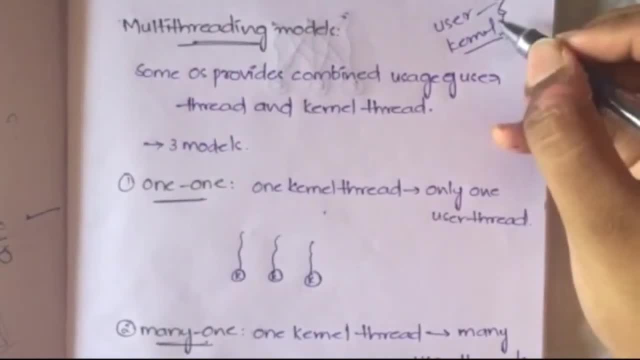 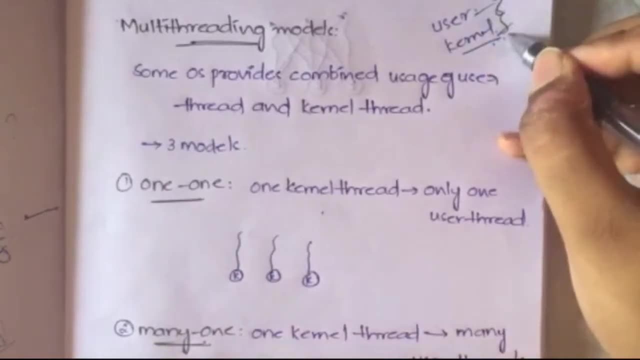 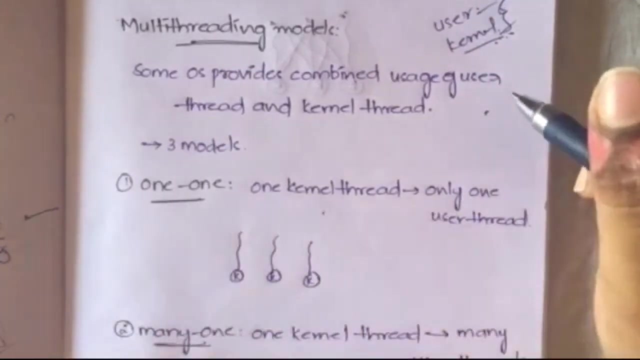 threads. both will be combined. sometimes one user and one kernel, or sometimes more than one user and single kernel. sometimes many users, many kernels. all those combinations will be happening. so we have three combinations. we have three models in multi-threading models. let us discuss about those three models in detail now. okay, the first one is one to one in one to one model, one user. this is a. 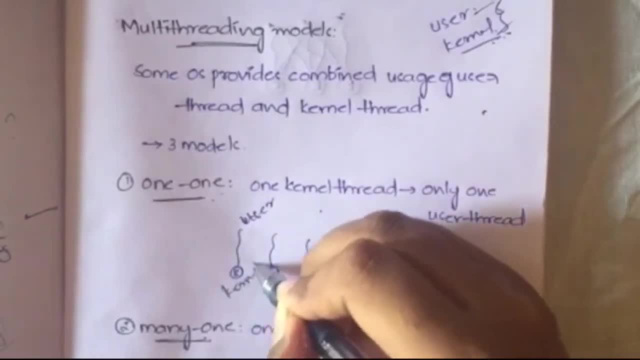 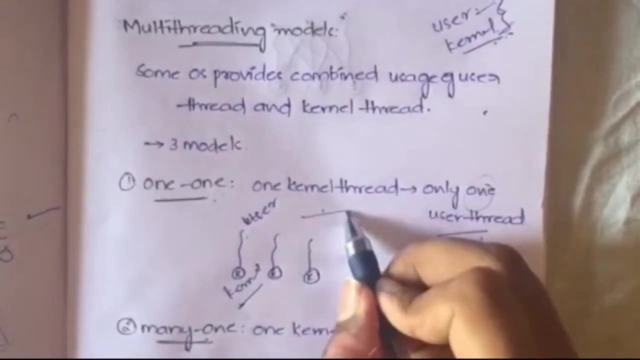 user thread. one user thread will be connected to one kernel thread. this is the kernel thread. one user and only one kernel. that means one user thread will be handled only by one kernel. that is, whatever the user operation is there, that will be done by using only one kernel thread. 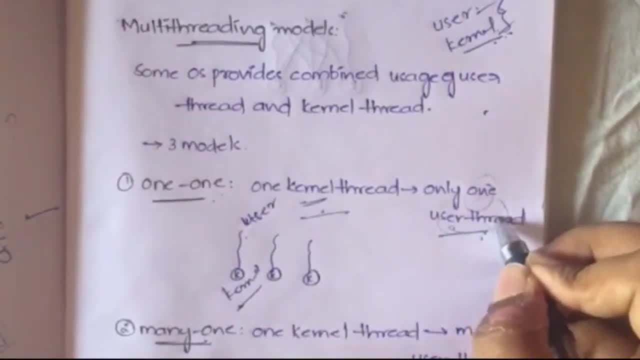 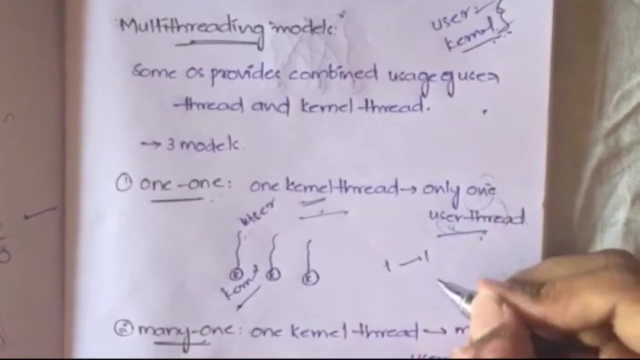 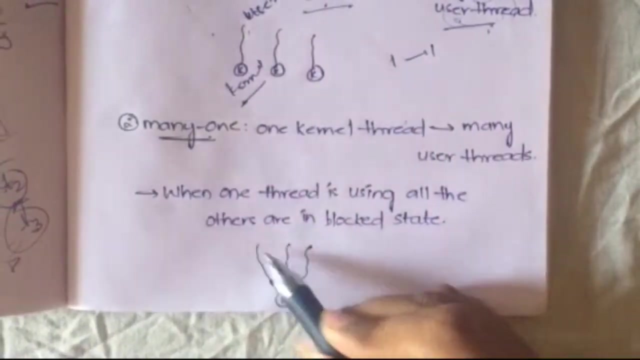 one kernel thread will handle only one user. that is about one to one model. one kernel, one user, that's it. it cannot handle more than one user. if two users come at a time, this one to one model cannot handle okay. second one is many to one model. here you have many user. 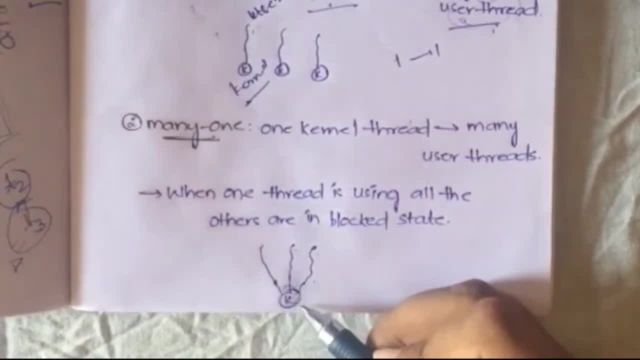 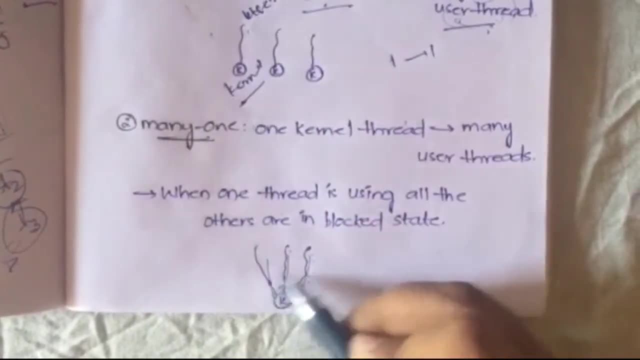 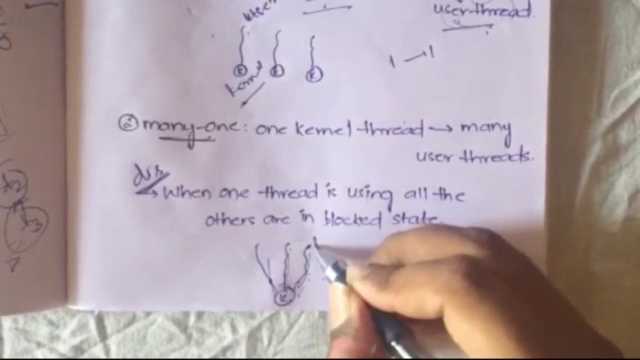 threads connected to only one kernel thread. that means one kernel thread will be handling many user threads. okay, here, what is the disadvantage that you have in this model is this is a disadvantage. the disadvantage is: suppose if this thread, this is a t3 thread, this is t2, this is t1, let's assume. suppose t3 is being handled by kernel. 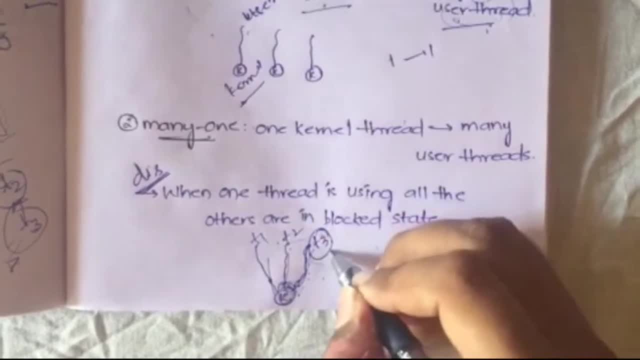 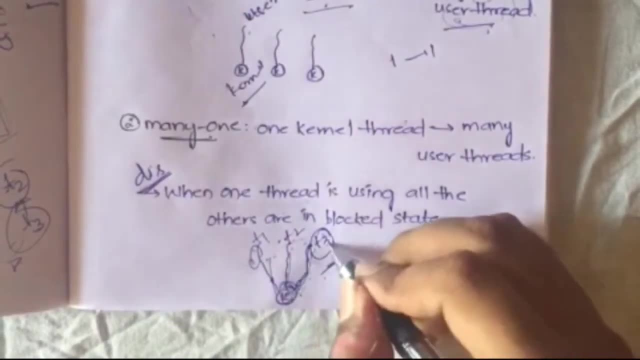 that means in kernel thread, kernel thread is operating the process, uh, the thread t3, then t1 and t2 has to go into the blocking state because one kernel thread can handle only one user thread at a time. so this is the disadvantage: when one thread is in execution, the other thread will enter. 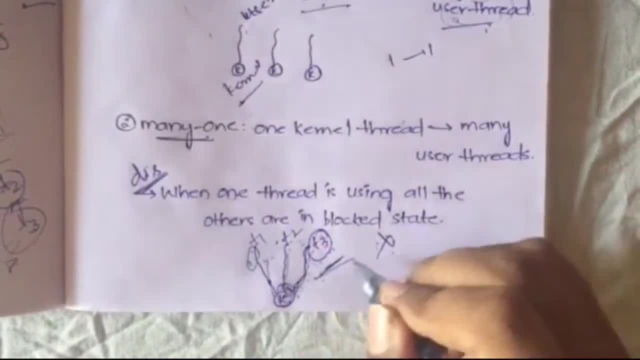 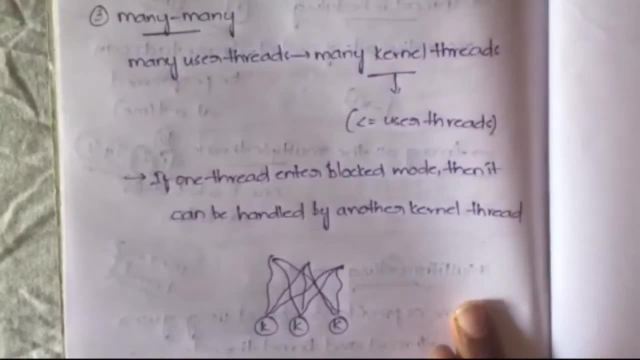 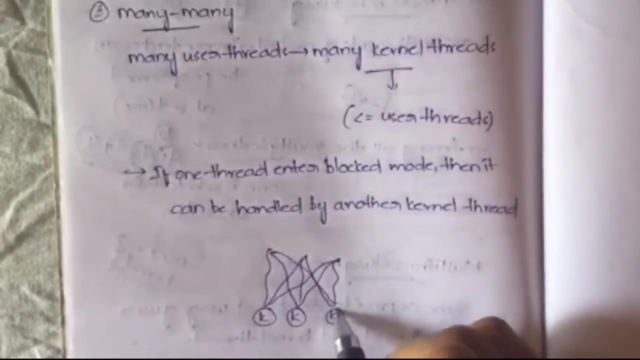 into the block state. that is the disadvantage that you have in many to one model. in many to one model, many user threads to a single kernel thread. okay, the last model that we have is many to many model. in many to many model, you will be having many user threads and also many kernel threads. you can do. 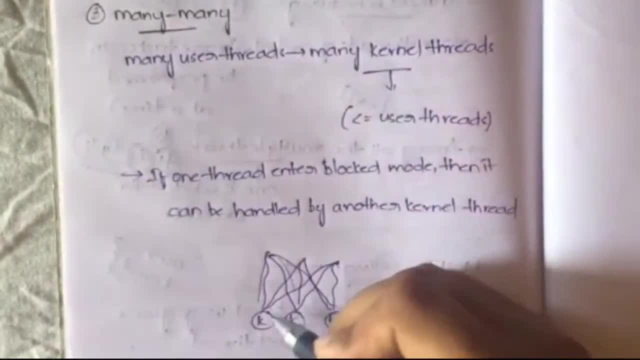 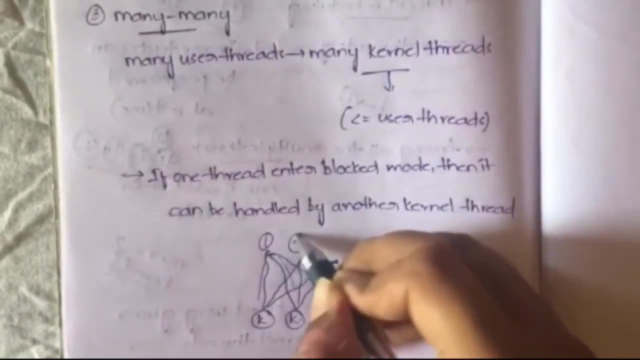 any number of combinations, okay, and when you are choosing this kernel thread, it should be less than or equal to number of user threads you are using. here you are using three user threads, so it should be less than or equal to three, but not more than three. okay, that is the condition that you have to. 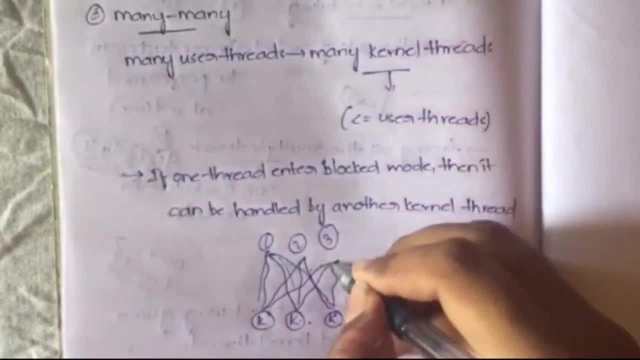 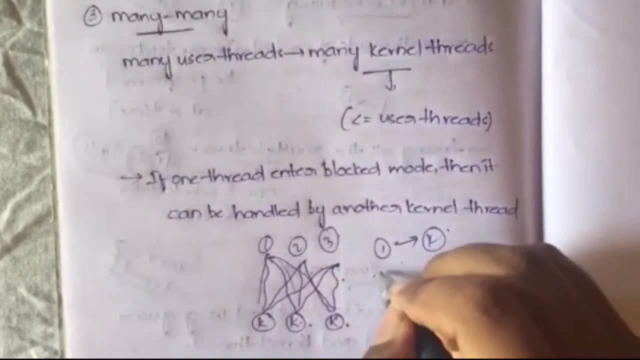 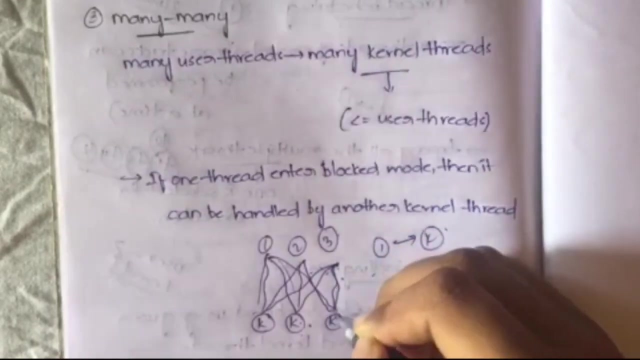 follow in many to any model and if in many to one model. if one pro one thread is being used by one kernel thread, then the other two threads has to be in block state. but here you don't have that problem because if suppose this is being used by this kernel, that means this kernel is handling this. 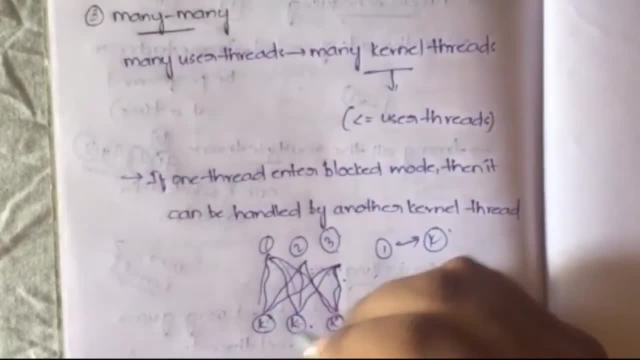 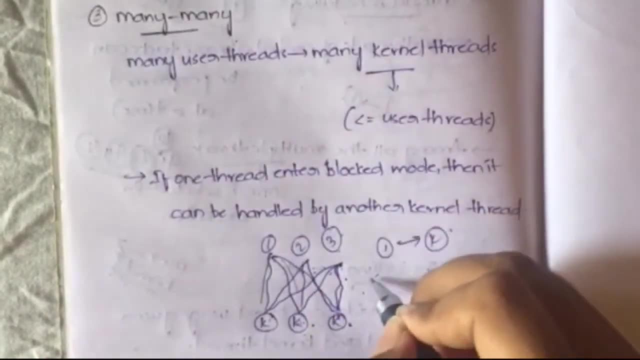 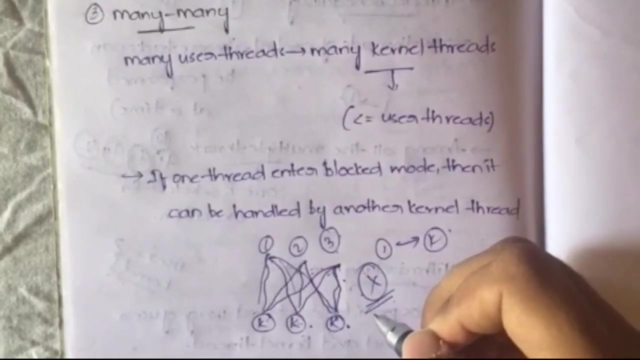 user thread, then the other threads can access to the other kernels. that is the disadvantage of this. sorry, that is. that is the advantage of this model. in many, to many model there is a no chance of blocking state. okay, this is about thread scheduling and the concept of threads and multi-threading models. multi-threading models: you have three. 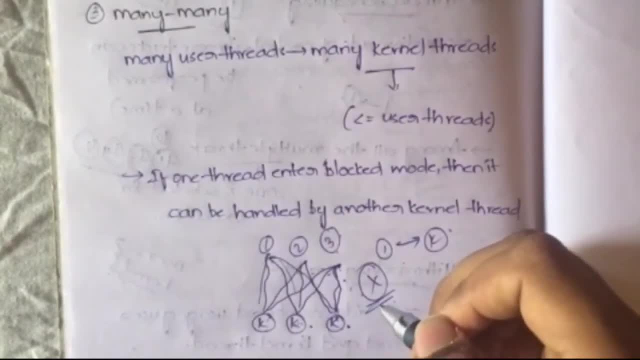 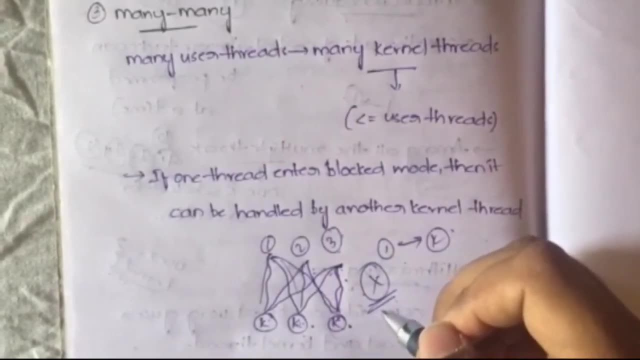 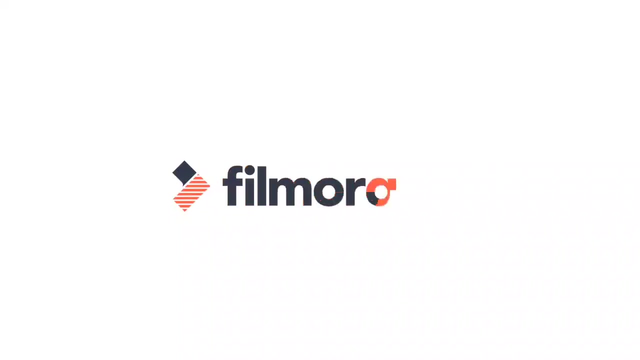 models: one to one model, many to one and many to many. in these three models you will be having number of combinations among user threads and also the kernel threads. okay, thank you so much for watching. i hope you enjoyed this video and i will see you in the next one. 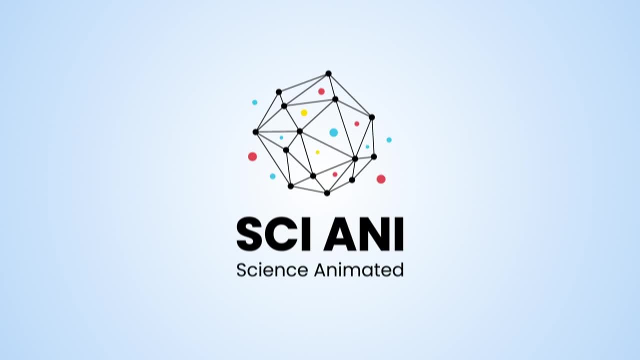 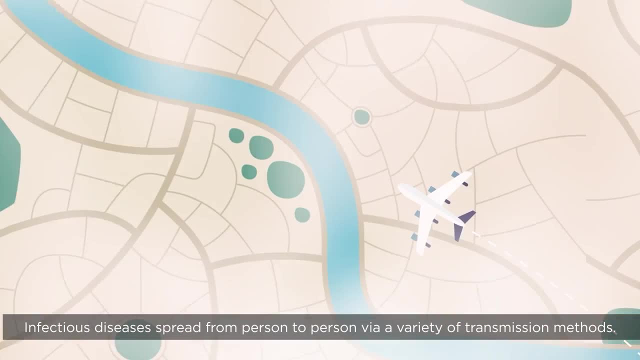 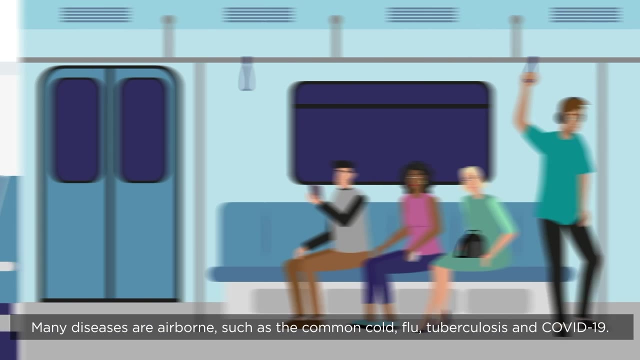 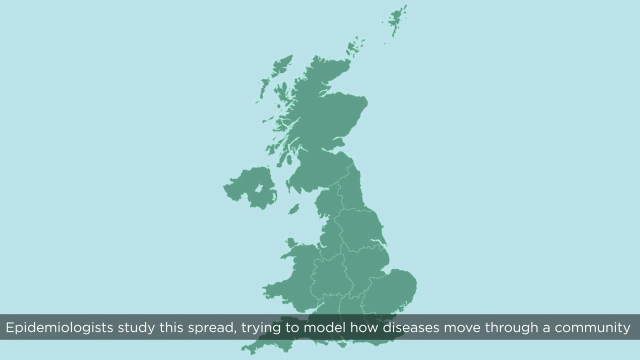 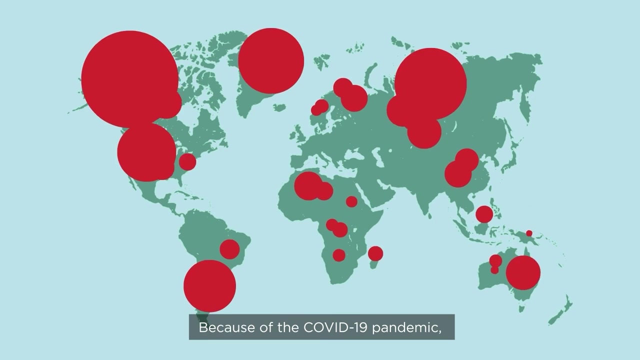 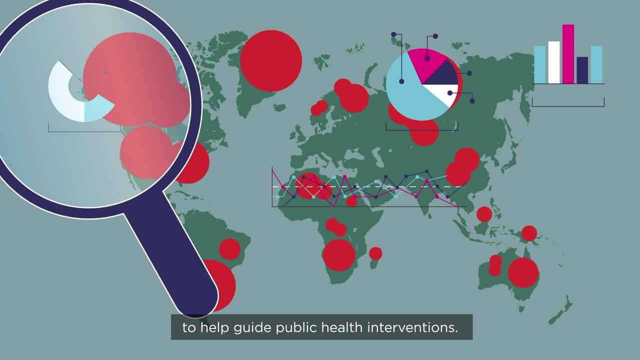 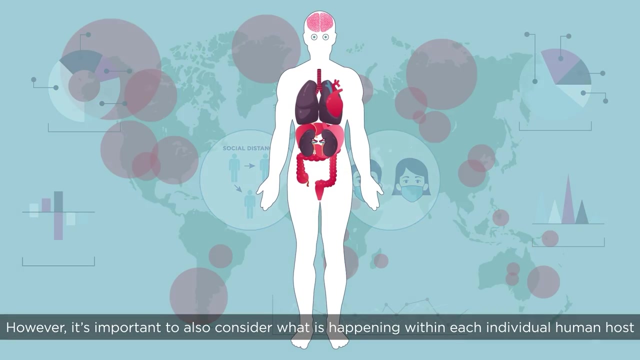 Transcription by ESO. Translation by —. Because of the COVID-19 pandemic, many people now understand how important mathematical models can be to help guide public health interventions. However, it's important to also consider what's happening within each individual human host and to model the dynamics there too. 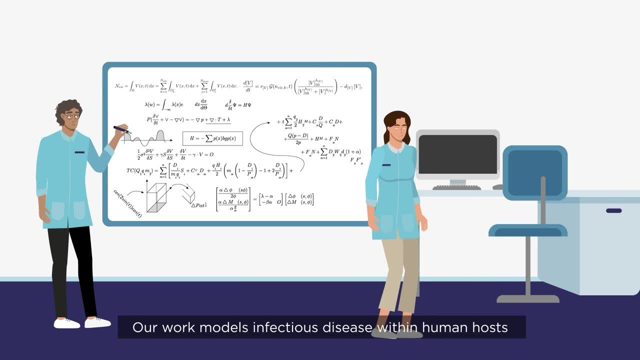 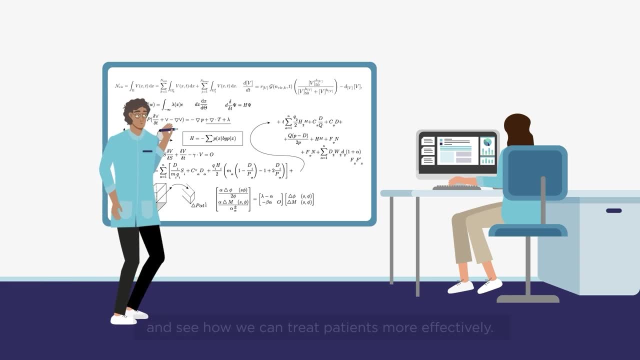 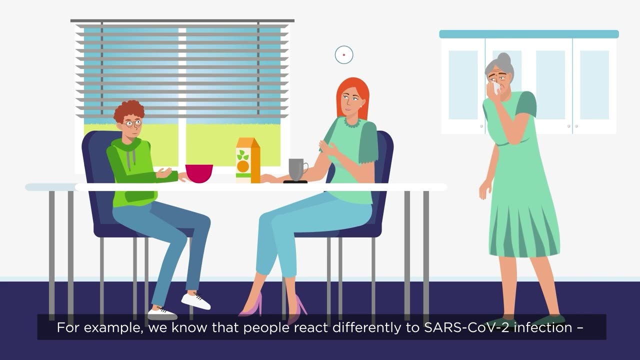 Our work models infectious disease within human hosts using individual-based mathematical models and differential equations, Helping to understand more about the infection and see how we can treat patients more effectively. For example, we know that people react differently to SARS-CoV-2 infection. 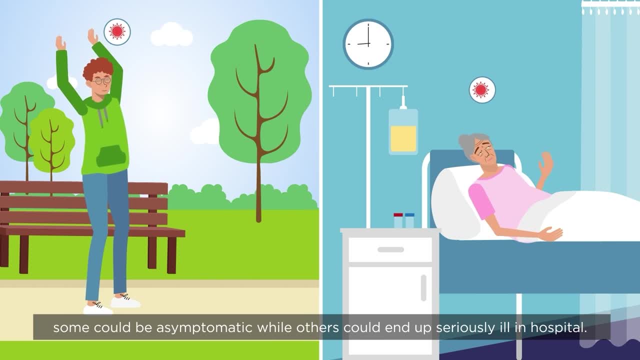 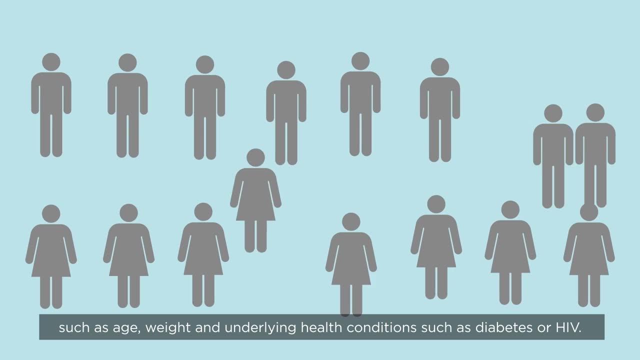 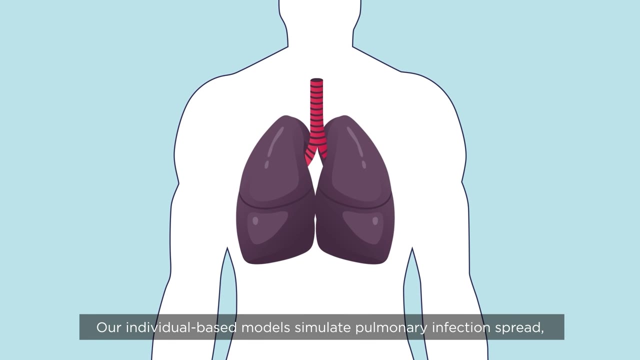 Some could be asymptomatic, while others could end up seriously ill in hospital. The differences in people's immunology can be affected by several clinical factors, such as age, weight and underlying health conditions such as diabetes or HIV. Our individual-based models simulate pulmonary infections. 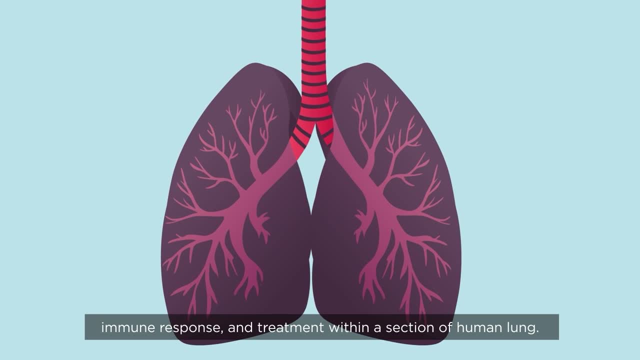 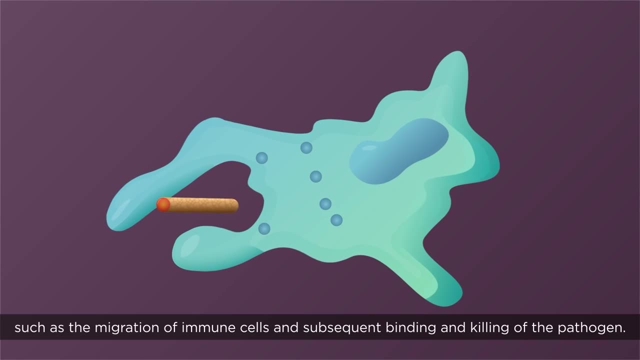 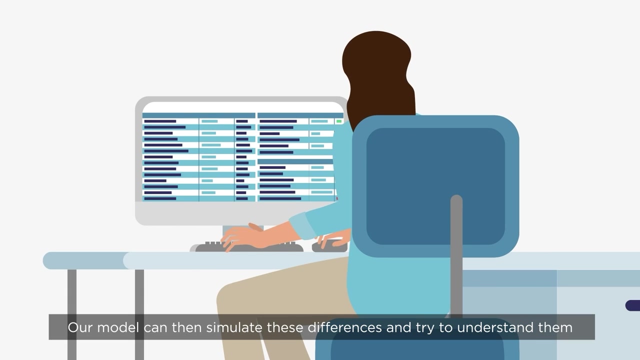 Infection, spread immune response and treatment within a section of human lung. The model contains discrete agents which model spatio-temporal interactions such as the migration of immune cells and subsequent binding and killing of the pathogen. Our model can then simulate these differences and try to understand them, with the goal of personalising patient treatment and improving their outcomes.